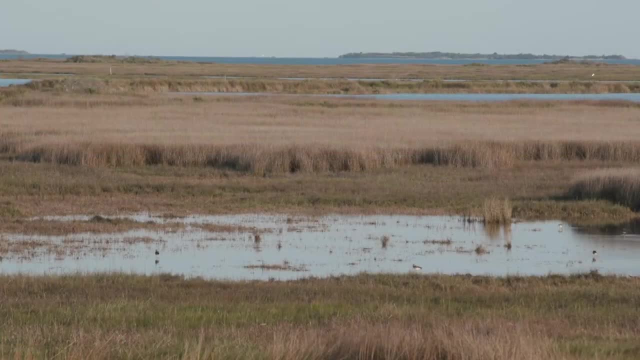 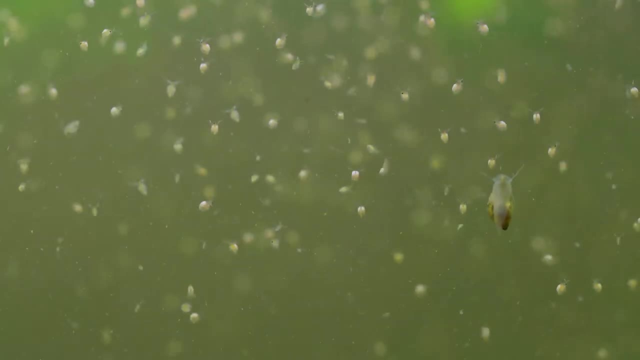 The Albemarle-Pamlico estuarine system consists of many different habitats, including marshes, oyster reefs, sandy beaches and grass flats, and each of these habitats provide for wildlife such as plankton, birds and fish. 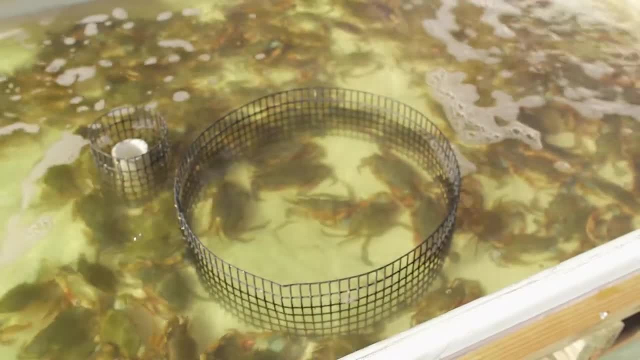 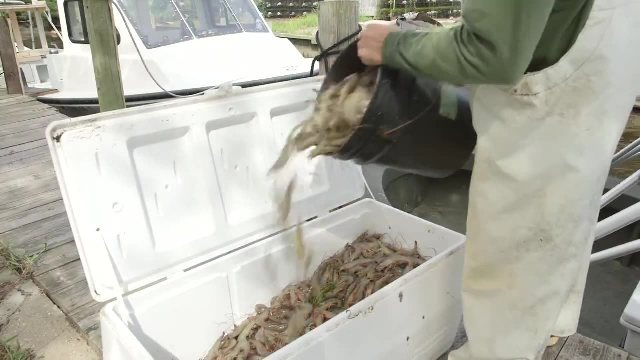 The estuary also plays an important economic role for the state of North Carolina. On a national level, estuaries are the nursery grounds for up to 75% of the seafood we catch. It is teeming with fish and shrimp targeted by the seafood industry, therefore providing 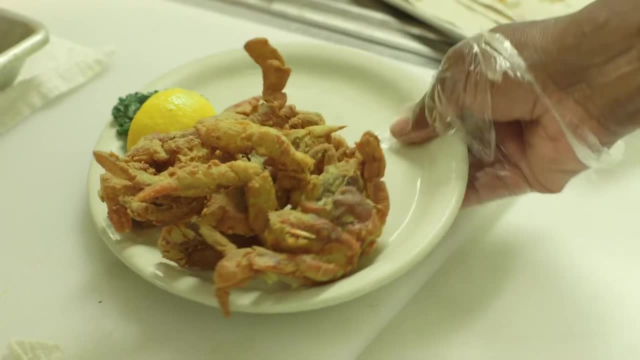 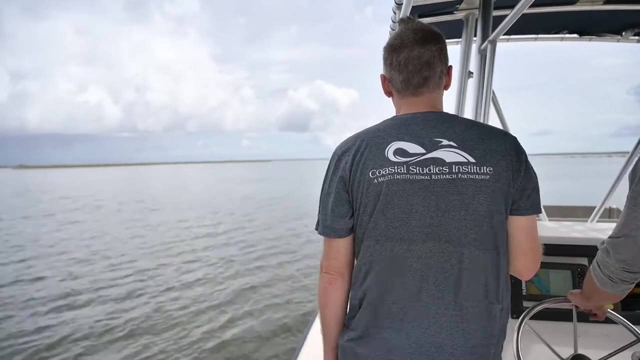 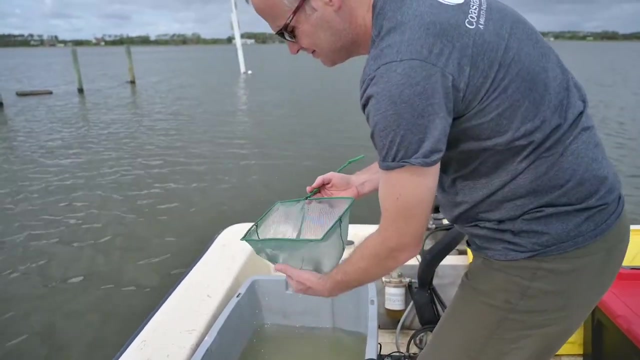 food and jobs for North Carolinians. Because the Albemarle-Pamlico is such an important ecological and economic resource, it is important we understand its system dynamics. Researchers at CSI are currently working to better understand important components such as the relationship between people and the estuary and how fish use the estuary throughout. 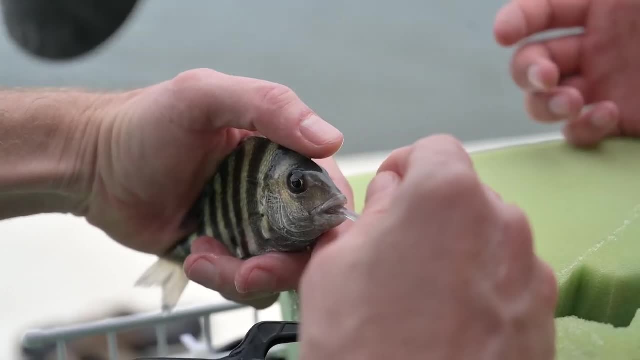 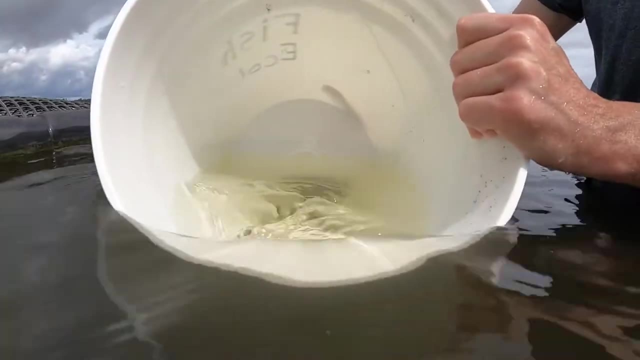 various life stages. Really, a critically important aspect of estuaries is there are distinct types of habitat in estuaries that do not occur in the ocean, And different species relate to each other. They rely on those habitats at different points in their life stage. 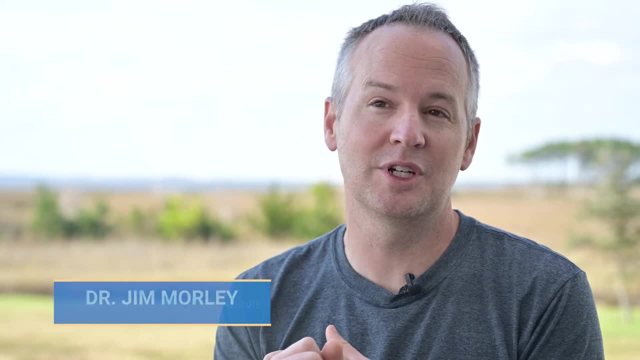 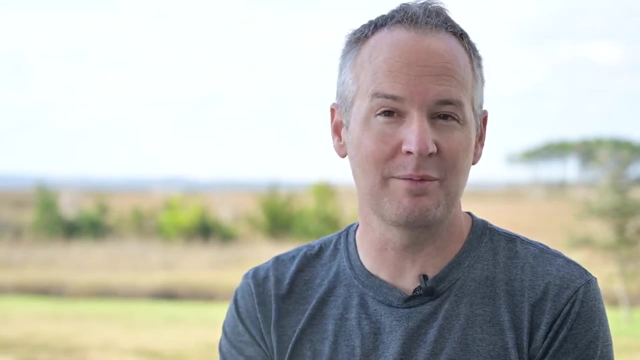 One of the reasons why they rely on these habitats is because they're effective areas for foraging. So not only do they provide protection against larger predators- and we're talking about smaller juvenile fish and shrimp- but they provide lots of food to eat and allow them. 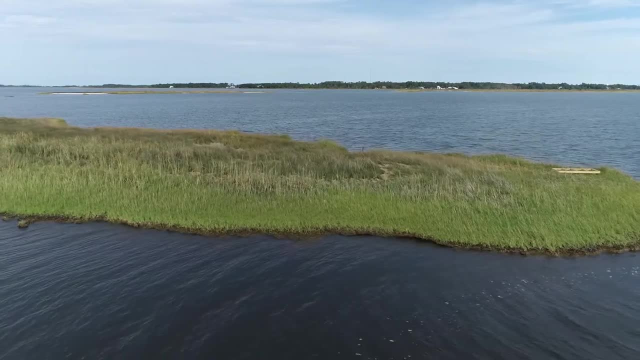 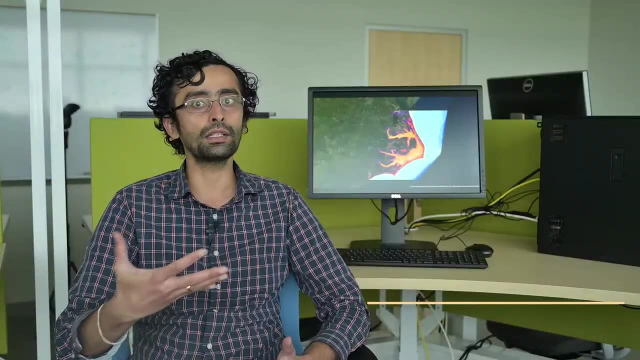 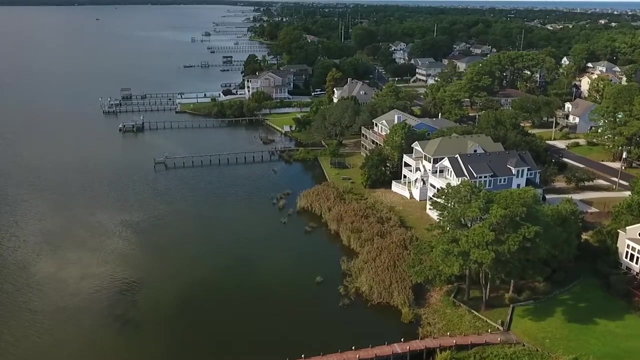 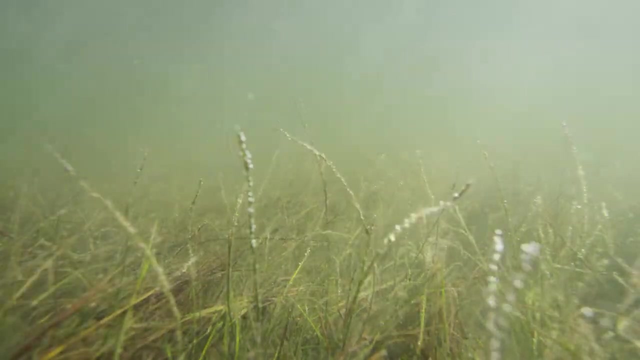 to grow, So that's critically important. Coastal estuaries are vibrant ecosystems, But they're also affected by the various pressures that they face, both in terms of human development, but also climate change and sea level rise. And when we lose these ecosystems, we don't just lose the ecosystems, we also lose the 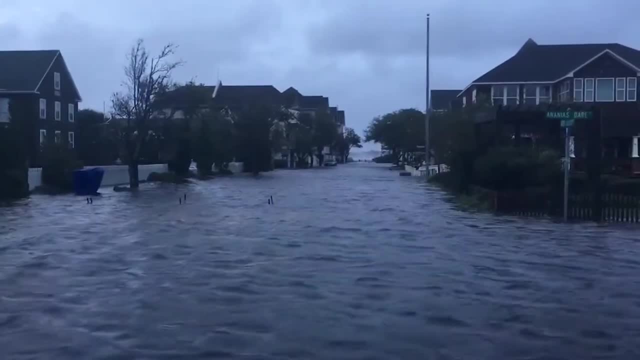 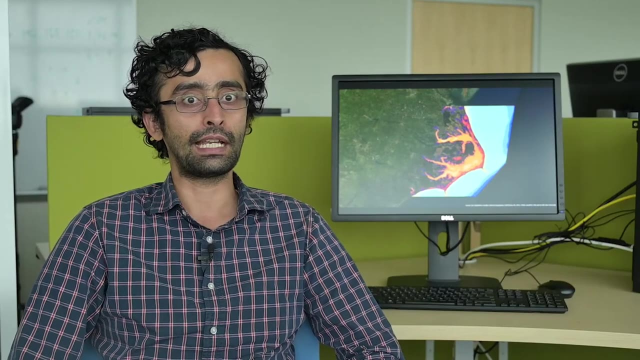 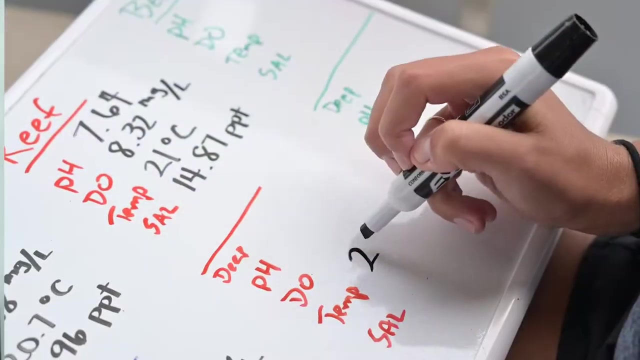 benefits that they provide to us, including protecting us from coastal flooding, for instance, when there's a storm. There are things that each of us, as individuals, can do to help protect our estuaries, especially who live close to these estuaries. One of them is to make sure that we reduce the.